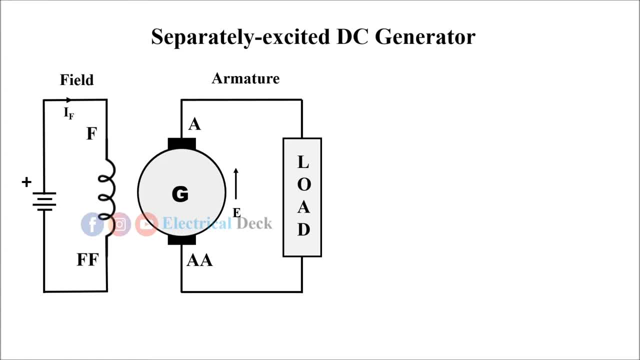 Here we can see that the excitation to the field winding is separate from the armature, Hence the generator is called as separately excited DC generator. The field winding of this type of generator consists of large number of turns with thin wire, So the resistance of the field winding is high. in order to limit the field current. 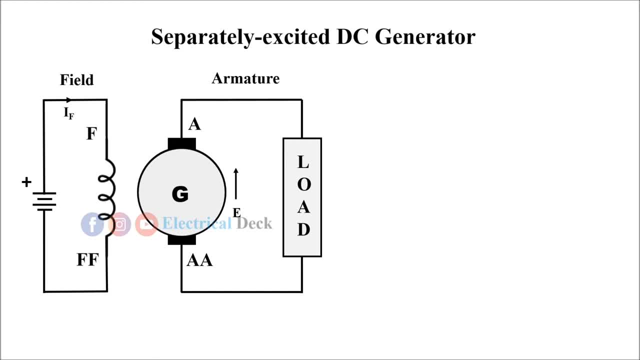 Now from the circuit diagram we can see that armature current I A is equal to load current I L. Therefore the terminal voltage V generated at the load is given by E is equal to V plus I A R A plus V brush. where E is induced emf, that is pi p n z by 60 A. I A R A is the armature winding drop. 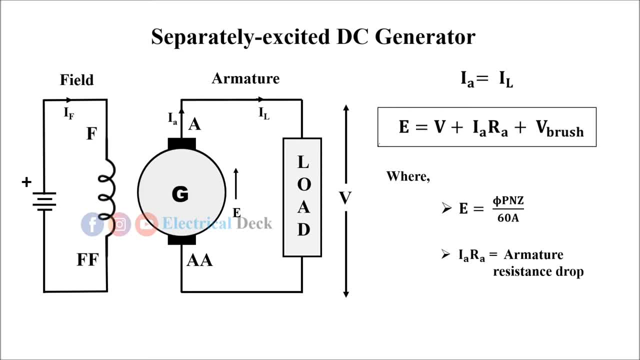 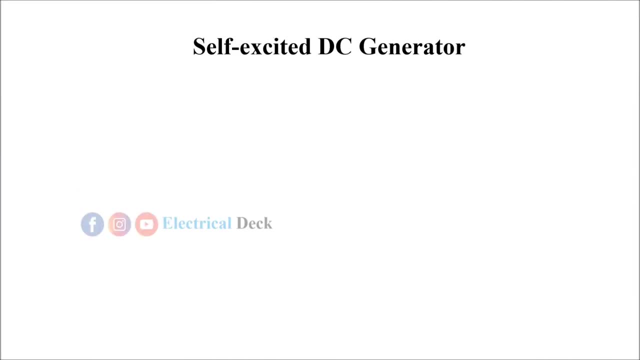 due to armature winding drop And V brush is called brush contact drop at the commutator. Generally, brush contact drop is negligible compared to other voltages, Hence it can be neglected. Now let us see the self-excited DC generator. In self-excited DC generator, field winding is supplied from the armature of the generator itself. 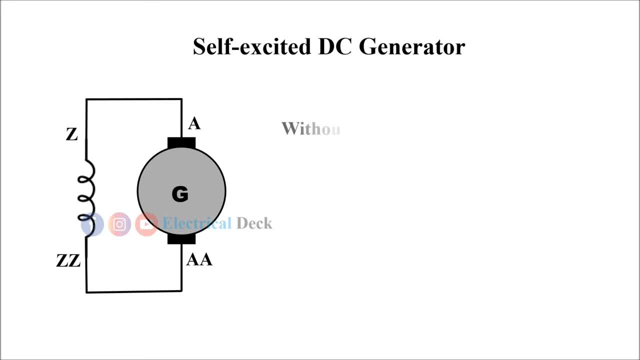 Here you may get a question that without generated emf field cannot be excited And without excitation there cannot be generated emf. Then how a self-excited DC generator works? The answer is residual magnetism by the field poles. Thus, when a generator started, the field poles posses some residual flux. 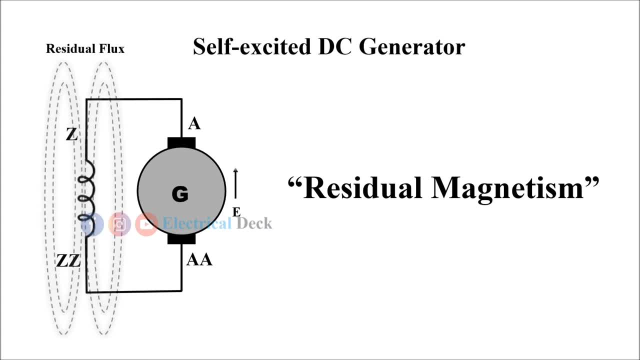 This flux develops small emf In the armature, Which in turns armature drives a small currents through the field winding. This further increases the amount of induced emf in armature. This process continues till the generator develops the rated voltage at the armature. 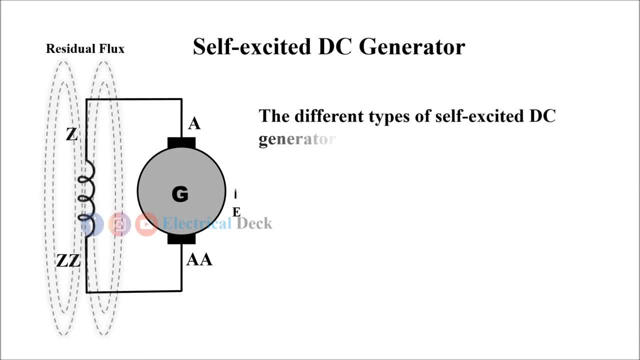 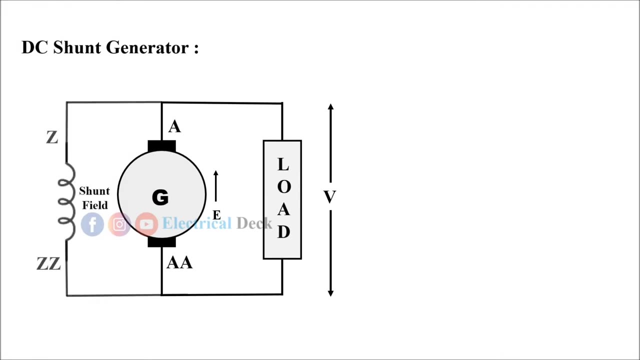 The different types of self-excited DC generators are DC shunt generator, DC series generator and DC compound generator. In DC shunt generator, the field winding is connected in parallel with the armature winding And the load is connected across the armature terminals. 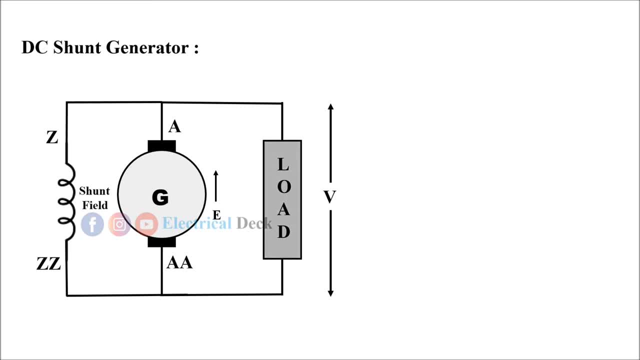 The field winding of DC shunt generator is similar to field winding of separately excited DC generator With large number of turns. Let RSH be the resistance of the field winding. Let RSH be the resistance of the field winding. Let RSH be the resistance of the field winding. 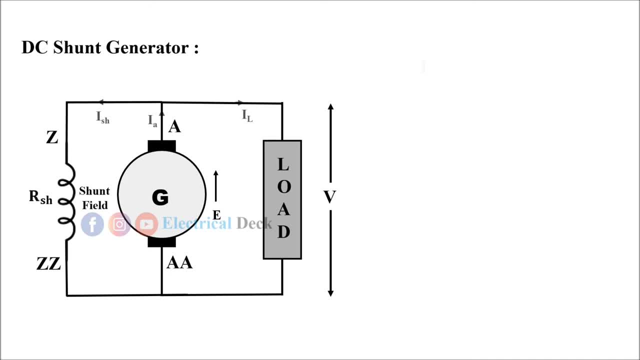 From the figure we can write that Armature current IA is equal to load current IL plus field current ISH. Here field current ISH is equal to V by RSH. Therefore the terminal voltage V generated at the load is given by E is equal to V plus IA, R A plus. 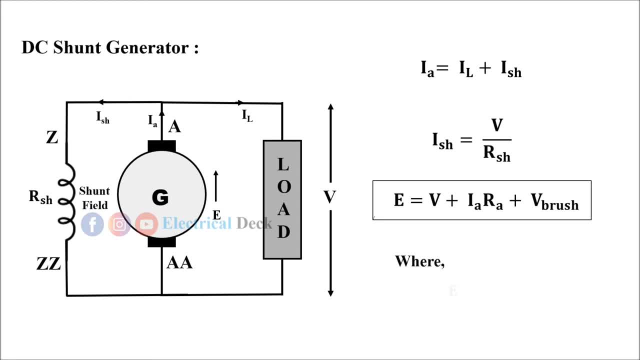 V brush where E is induced emf, Let RSH be the resistance of the field winding. That is pi p n z by 60 A. Here also the induced emf E requires to supply the armature winding. drop I A R A due to armature. 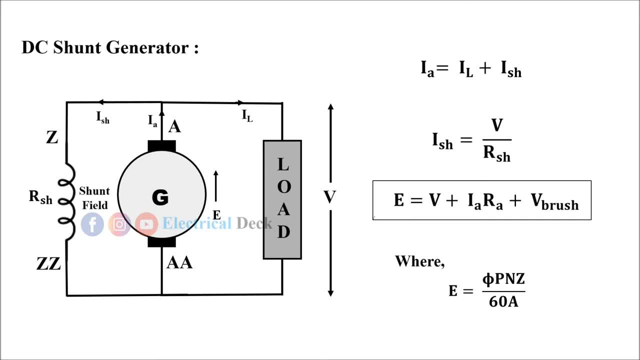 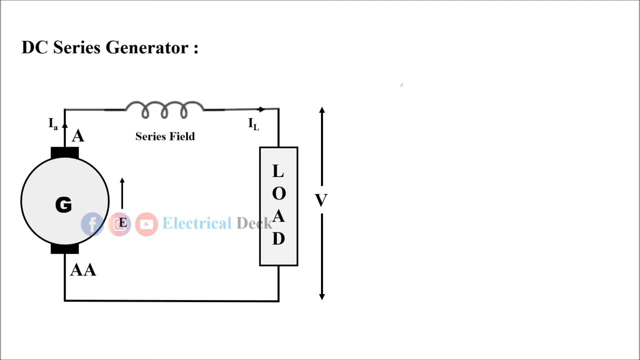 resistance and brush contact drop at the commutator. When the field winding is connected in series with the armature winding while supplying the load, then the generator is called DC series. Then the generator is called DC series Field winding, in this case denoted as Y and YY. 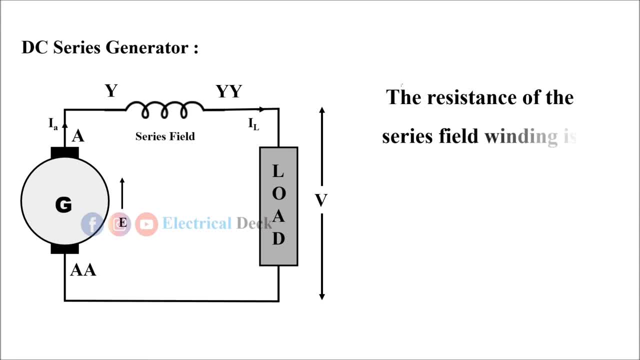 The resistance of the series field winding is very small, With less number of turns and thick cross section of wire. Let RSH be the resistance of the series field winding. From the figure we can see that All armature field and load carry the same currents due to series connections. 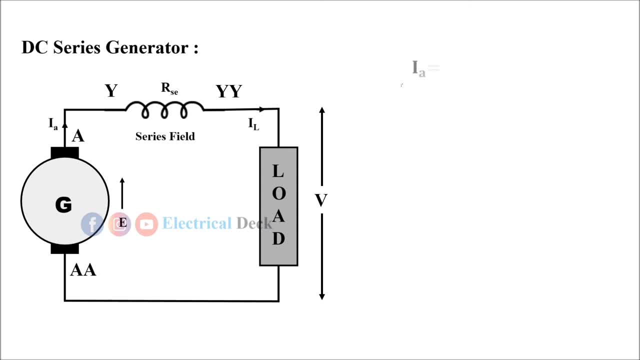 Therefore, armature current I A is equal to load current I L is equal to field current I SE. Now the terminal voltage V generated at the load is given by E is equal to V plus I A, R, A plus I, S, E, R, S, E plus V brush, where E is induced, emf. 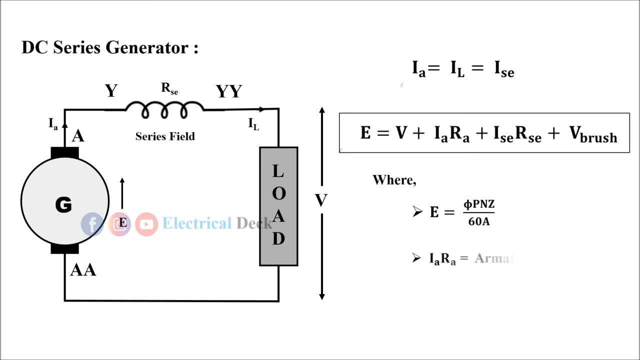 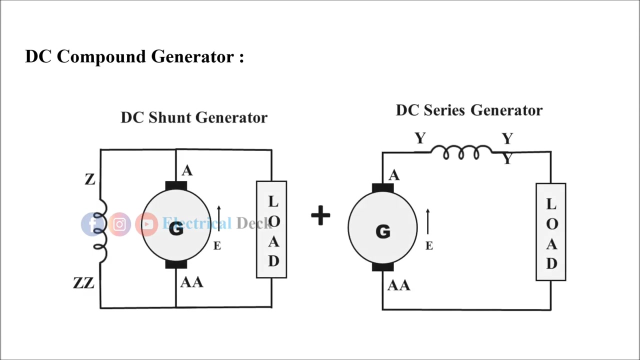 That is pi p n z by 60 A. Here, in addition to the drop, I A R A induced emf. as to supply voltage drop across the series field winding also, That is I S E R S E. The DC compound generator is the combination of both DC shunt and series generators. 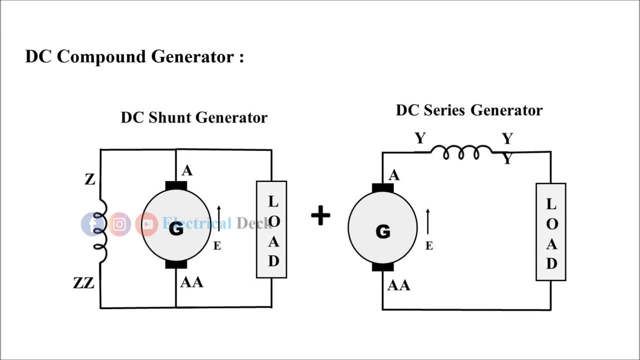 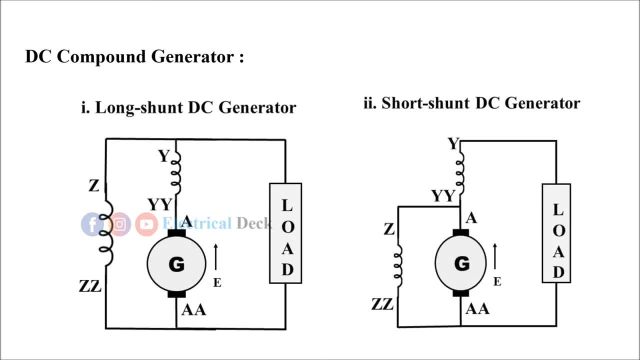 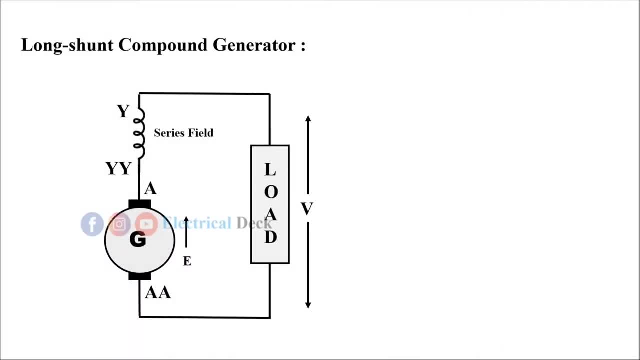 They are long shunt compound generator and short shunt compound generator, DC shunt and series generator. In long shunt compound generator the shunt field winding is connected across the series field winding. In this generator, series field current is equal to armature current. 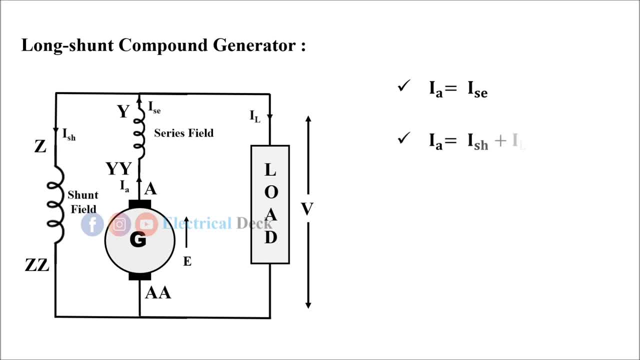 And armature current is the sum of shunt field current and load current. The shunt field Shunt field resistance I sh is given by load voltage V divided by shunt field resistance R sh. Therefore the voltage equation for long shunt compound generator will be same as series. 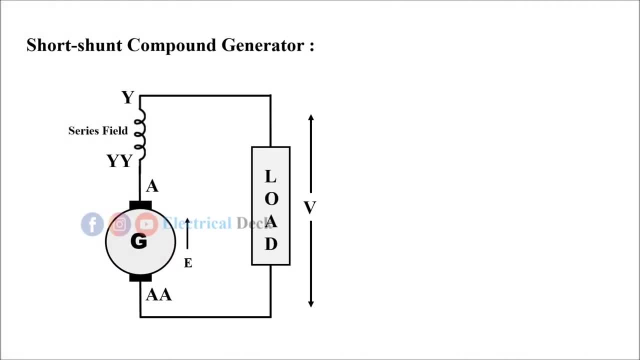 generator, In short shunt compound generator. the shunt field winding is connected only across the armature winding. In this generator, series field current is equal to load current and armature current is the sum of series field current and shunt field current. 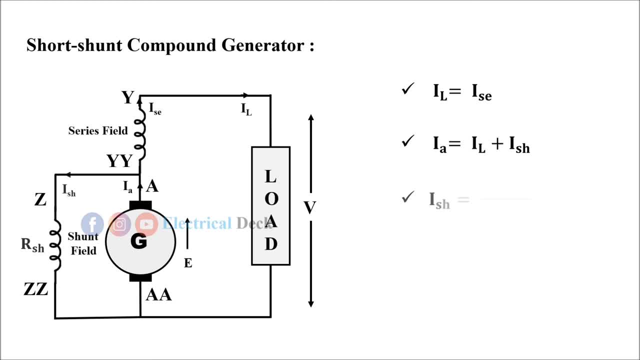 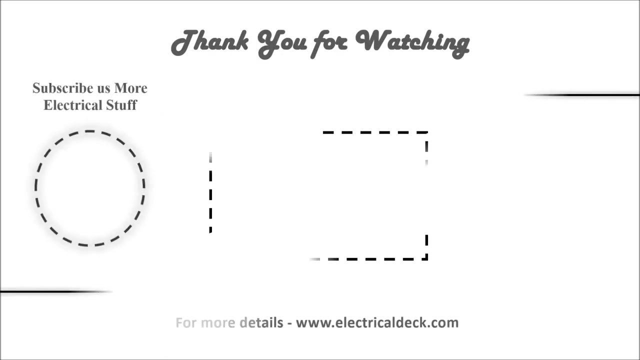 Here the shunt field resistance I sh is given by emf induced E without armature resistance drop, divided by shunt field resistance R sh. Here also the voltage equation for DC short shunt compound generator will be same as series generator. Thank you for watching video. 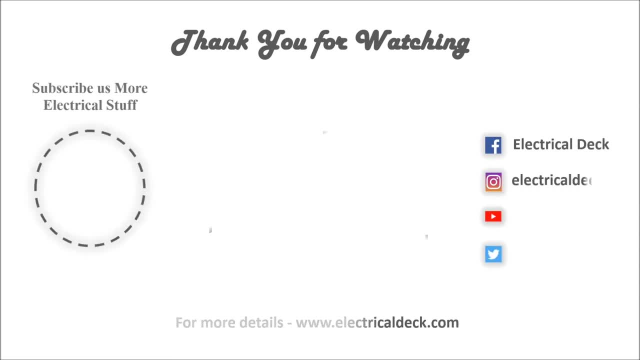 See you soon again, And don't forget to subscribe us for more electrical stuff.